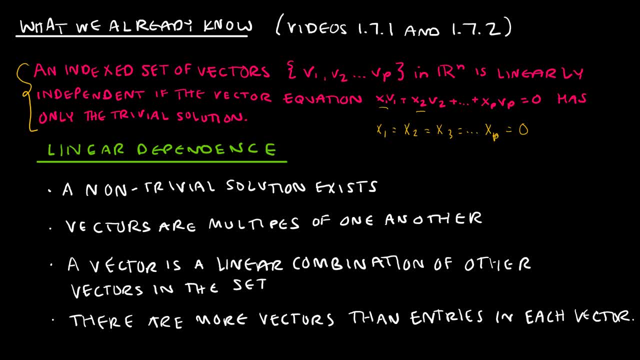 which is what the x values would be in this case, would have to be equal to 0. So if it's linearly dependent, then obviously this would not be true. one of our scalars would have to not be 0, and that would be a non-trivial solution. 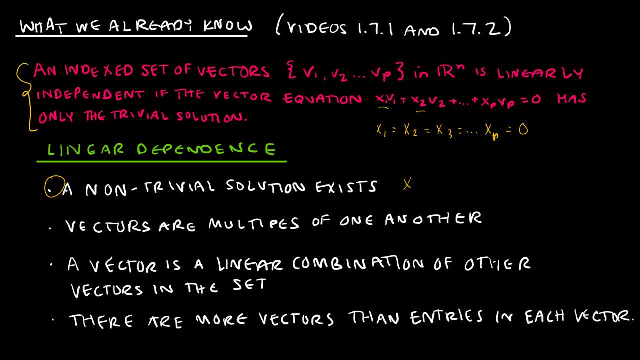 exists. So say x, I don't know. n would have to be not equal to 0 in order for a non-trivial solution to exist. If vectors are multiples of 1.7u, then the linear青ITY and the rationalization agreement for it to only have the trivial solution is one to zero If vectors are multiples of 1.7n. 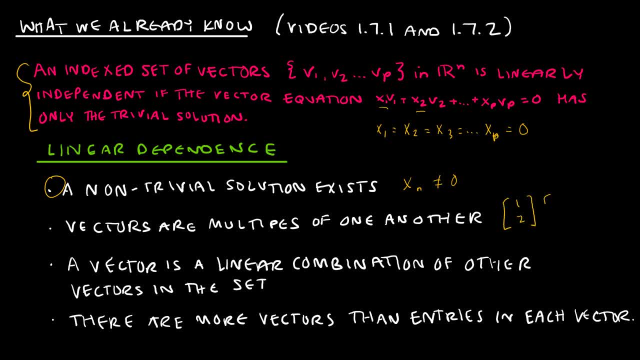 one another. So say I had 1,, 2, and then 2, 4.. These are multiples of one another and therefore are linearly dependent. If a vector is a linear combination of other vectors in the set, so let's stick with. let's say I have 1,, 2, and this one is negative- 3, 4.. 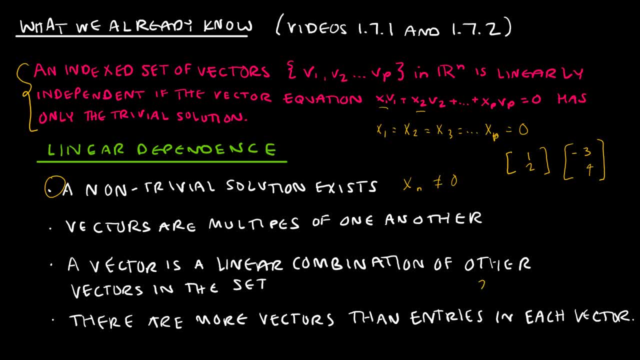 And then let's say if I had 2, we'll call this v, we'll call this w. Let's say I had 2v minus w, That would be 2 times 1 is 2 minus negative, 3 is 5.. And then 2 times 2 is 4 minus. 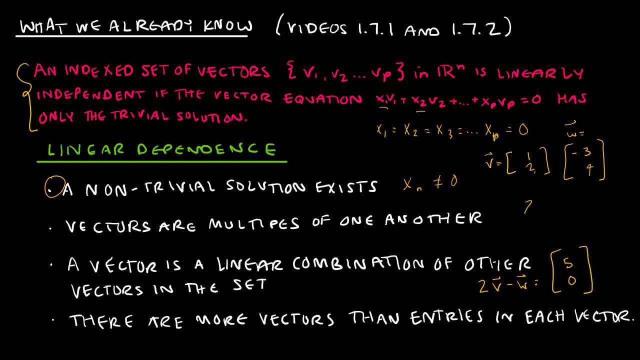 4 is 0. So let's say vector z was 5, 0. Well then, for sure I know that this is linearly dependent, because I can take a combination of vectors v and w to arrive at z. So if it can be written as a linear combination of other vectors, 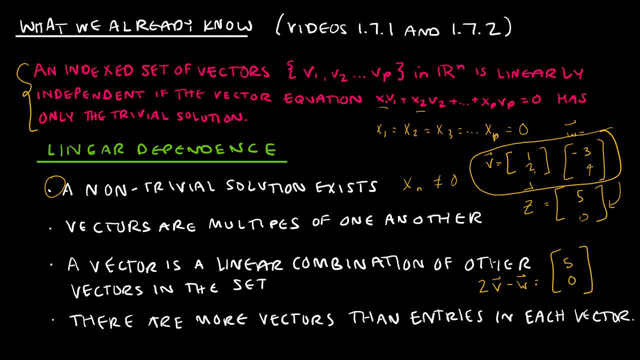 it's linearly dependent. And then of course there are more vectors than entries in each vector, which again, my example- I just did, the v w z example- would also be linearly dependent based on this. So if I went through any of that too quickly, go back to videos 1.71 and 1.72.. Otherwise, 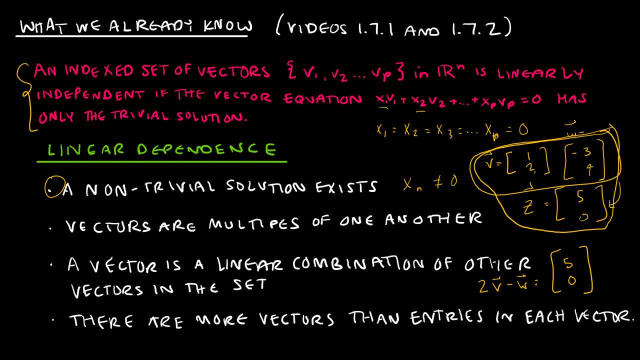 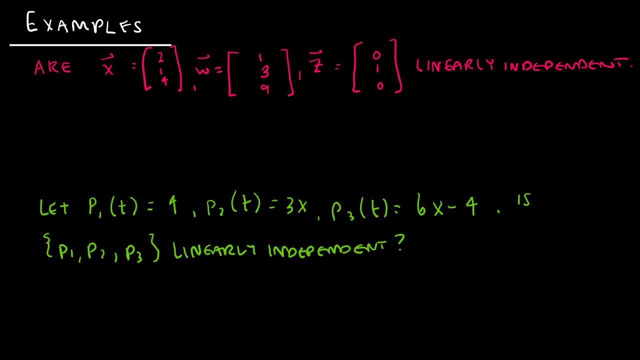 let's move on to the new stuff in this section. Let's look quickly at two examples of linear independence. The first should look familiar. We haven't done this again, but let's look at the first one. I haven't done this exact question before, but we've done questions like it. 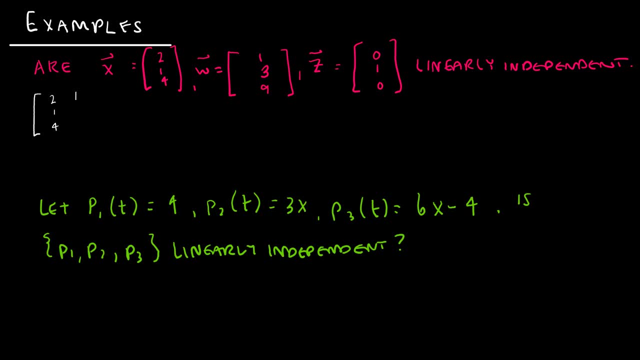 I'm asking if these three vectors are linearly independent. And when I have three vectors with three rows, I can't use one of my shortcuts. I have to do it the long way. Keep in mind that this is equal 0, 0, 0.. That's essentially what we're doing, is we're trying to determine linear. 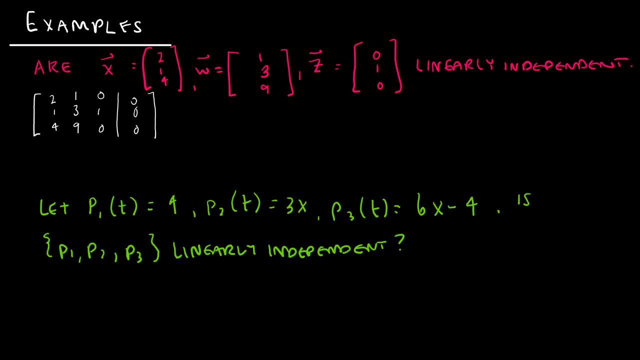 independence based on if we have a free variable or if we have only the trivial solution. So, continuing with row operations, I'm going to take half of the first row, So that's 1, 1, half 0, 0.. And that's all I'm going to do for that first step. And I've got a pivot right where. 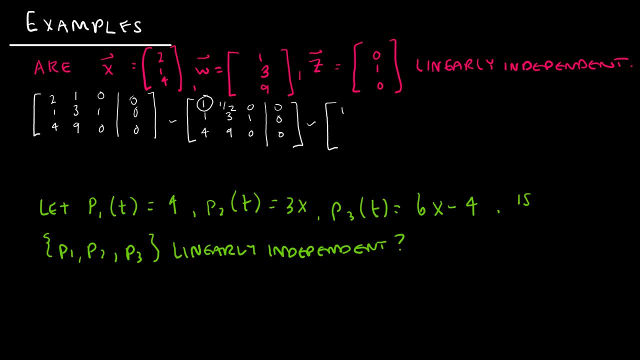 I want it. I'm going to make zeros below that. So I've got 1, 1, half, 0, 0.. And then I'm going to just subtract row 1 minus row 2 to give me 0, to give me negative 5 halves, to give me negative 1,. 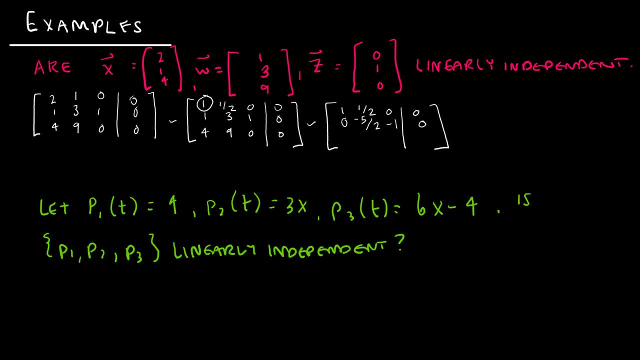 0.. And I'm going to take negative 4 times that first row. So negative 4 plus 4 is 0.. Negative 2 plus 9 is 7.. 0 plus 0 is 0.. So I have this pivot and I have it as a 1,. 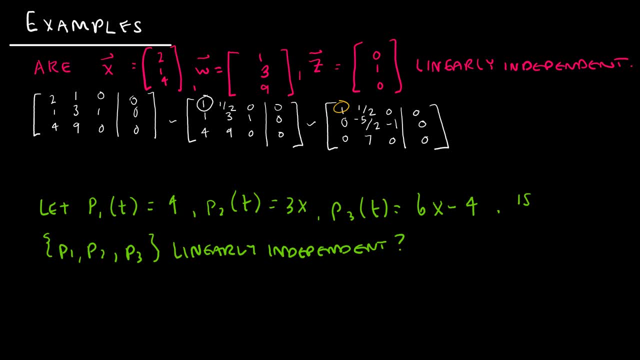 which is what I want. Now I'm going to get to the negative 5 halves to be a 1.. So 1, 1, half 0, 0.. I'm going to take everything times negative 2. fifths: 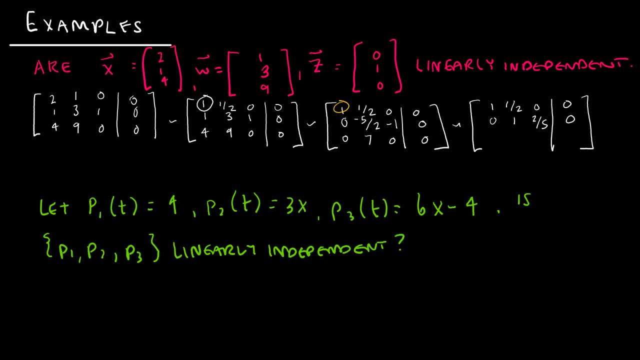 which gives me 0, 1, 2 fifths 0. And then 0, 7,, 0, 0. And then I will continue, because now I've got pivot pivot, And if I continue and you might be saying don't continue, we already know the. 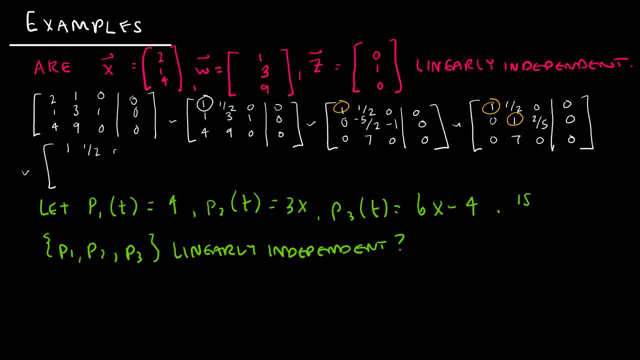 answer, but that's okay, Let's keep going: 1, 1, half, 0, 0, 0.. Oops, I shouldn't have done that yet The first row. I'm going to take the second row times negative 1 half and add it to the first row. 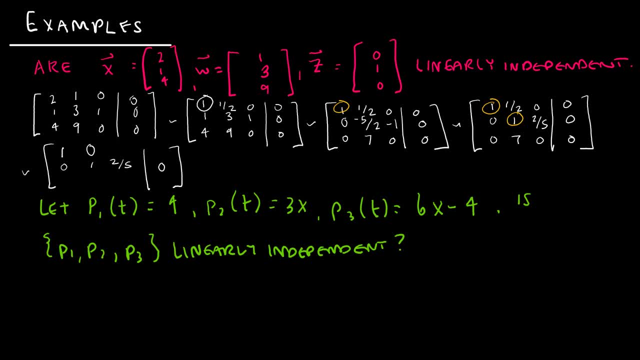 So that gives me 1 and 0, which is what I want, And then 2 fifths times negative. 1 half is negative 1 fifth. And then in my last one I'm taking negative 7 times the second row and adding it to. 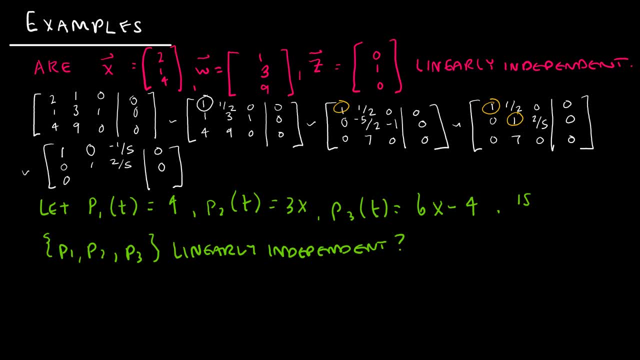 the third row. So that gives me 0, and that gives me 0, and then negative 14 fifths and 0. And again they're just asking for linear independence or not. So it doesn't ask me to actually find the solution, But what I know now is I've got a pivot here. I've got a pivot. 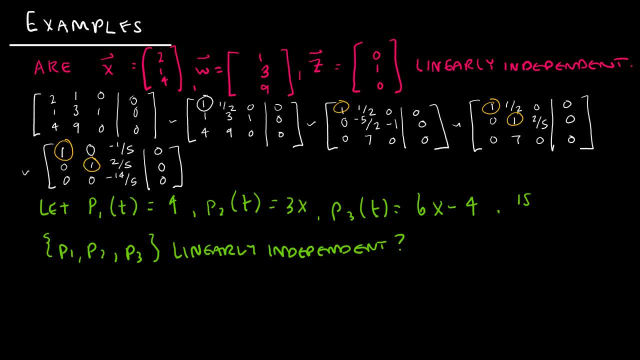 here I could continue my row operations to find the 0,, and essentially that would be the very, very next one, So I could have получается with an idol Namen, and then the next thing I'm going to plan is I would have 0, 1, 0, 0, 0, 1, 0, 0, 1.. 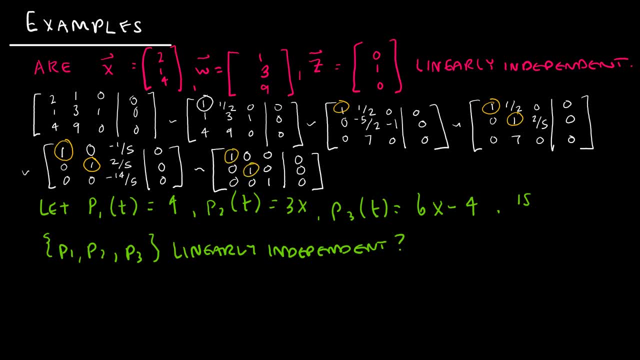 I'm not going to do the row operation, so make that happen, But you can imagine that they would be fairly straightforward. And notice, I end up with the identity matrix on the left side, which means that I don't have any free variables and therefore the only solution to a x- e equals too zero- is the trivial solution. 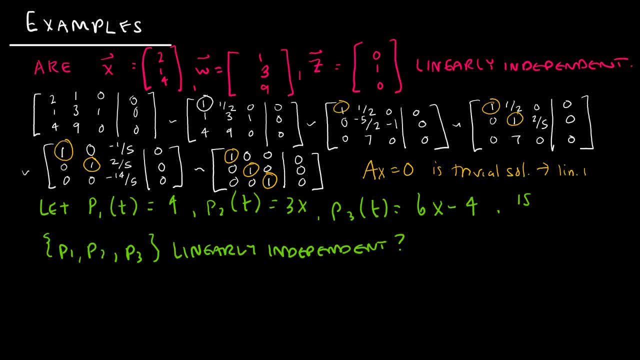 for this is linearly independent. Good, Let's look at an example we've never seen before which is dealing with polynomials. We talked a little bit about polynomials before, and now I'm trying to determine linear independence on those polynomials. So I have 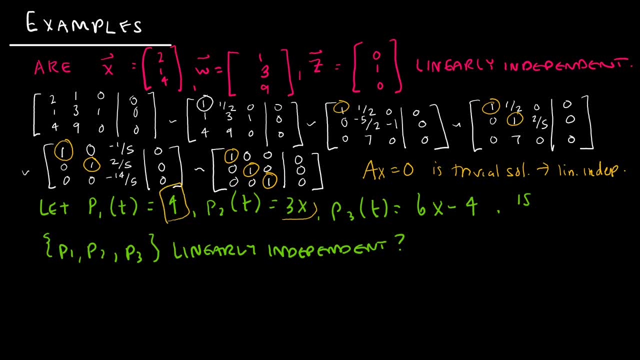 a polynomial of just 4, then I have a polynomial of 3x, and then I've got a third polynomial of 6x minus 4.. Again, we haven't looked at one like this, but what we can do is make it look kind. 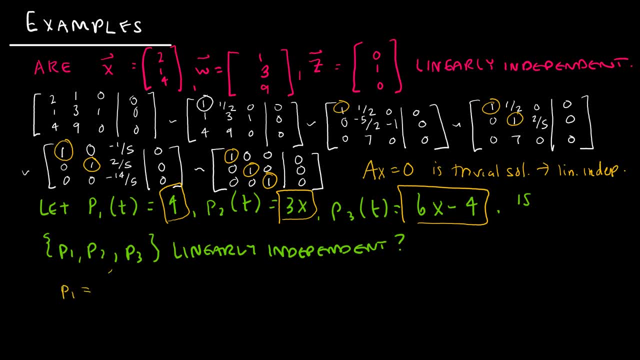 of like what we've seen before. So I can say p1 has 4 in the constant row and 0 in the t row or x row. That should be. yeah, we'll stick with it. These should be t's instead of x's, but you get. 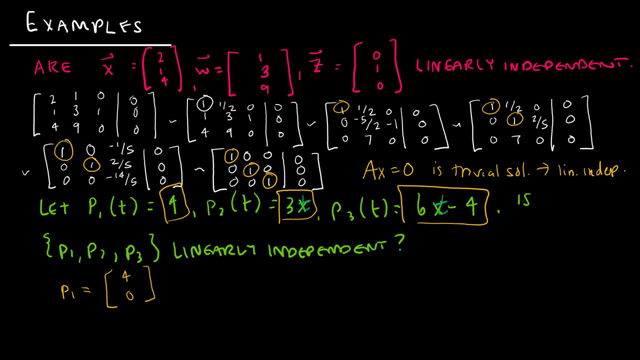 the idea, And so p2 could be rewritten then as 0 constant, 3 in the t1, and p3 could be rewritten as negative. 4 in the constant and 6 in the t1 row. And so then the question is: is one of these a? 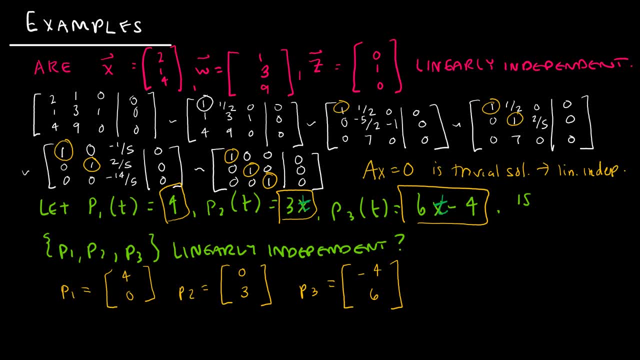 multiple of another, or could I write one as the linear combination of another? And in fact I can. I could write p3 as negative p1,, which would make it that negative 4, plus 2p2.. And if I did that I would. 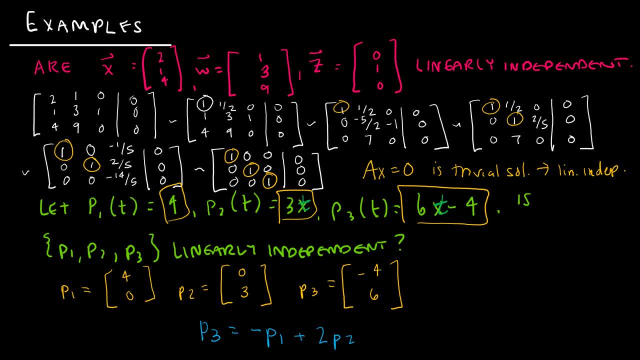 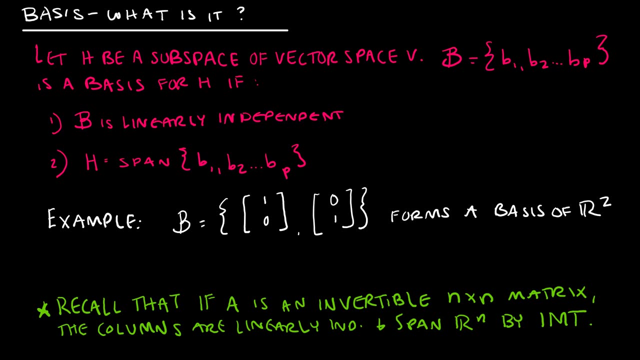 end up with p3. So, because p3 can be written as a linear combination of p1 and p2, these are linearly dependent. So now that we have reviewed what linear independence is all about, let's talk about what we really want to learn about. 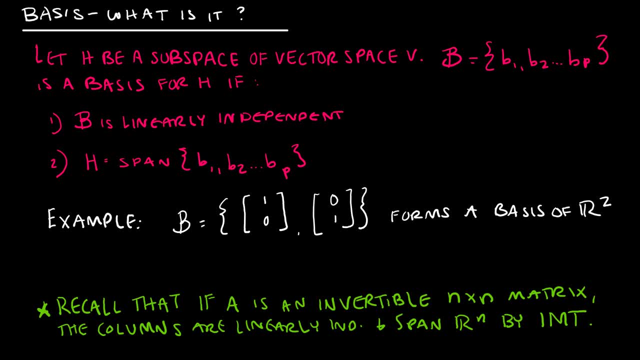 which is basis. So what exactly is a basis? Well, if we let h be a subspace of vector space v, then our basis b1, b2 through bp, is a basis if b is linearly independent, which is what we just. 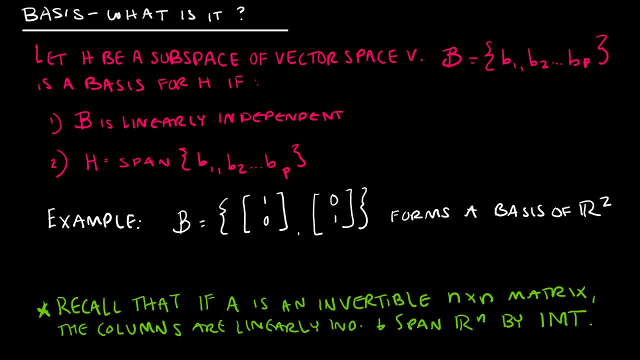 reviewed how to determine that. And if h, which is the subspace spans, h, is the span of f, of f, of f, of v, b, essentially of the basis. So, for example, if I have vector 1,, 0 and 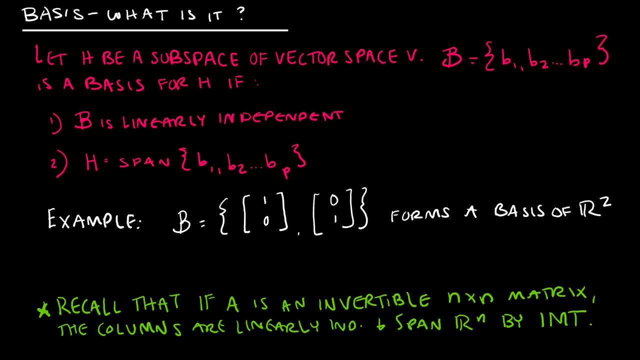 vector 0,1,. these form a basis of r2, and the reason for that is obviously those two vectors are linearly independent. One is not a multiple of the other, and those would span all of r2, because I could get to anywhere in r2, by some linear combination of those two vectors. So 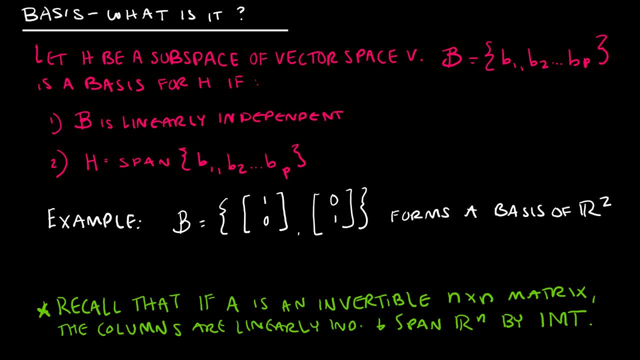 therefore, those two vectors are a basis of vector v. okay, B, alpha term, b, kw, omega i找им of R2.. Also, I want you to recall, as we're going through some examples, that if A is an invertible n by n matrix, then the columns are linearly independent and they span Rn by the invertible. 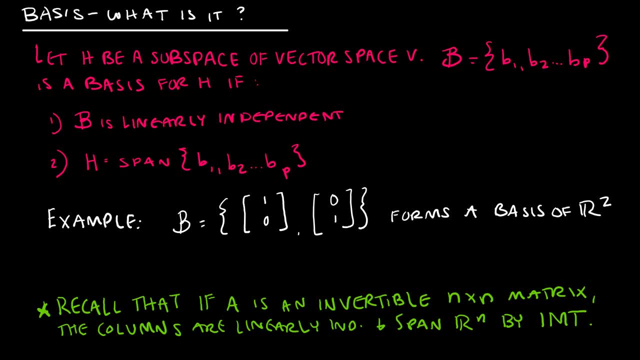 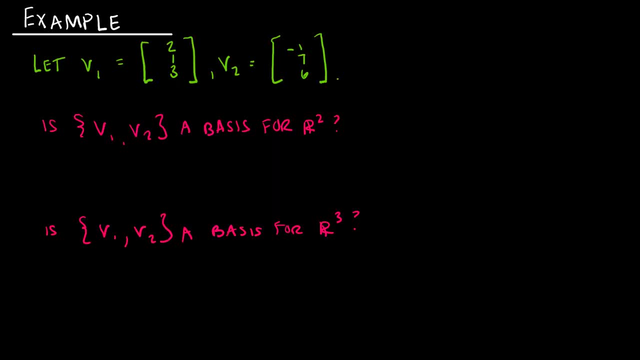 matrix theorem that we just learned about. So let's take a look at some examples. In this example I have V1 and V2 and asking if those two vectors, the set of those two vectors, form a basis for R2 or for R3.. So for R2, hopefully this one is pretty apparent- V1 and V2. 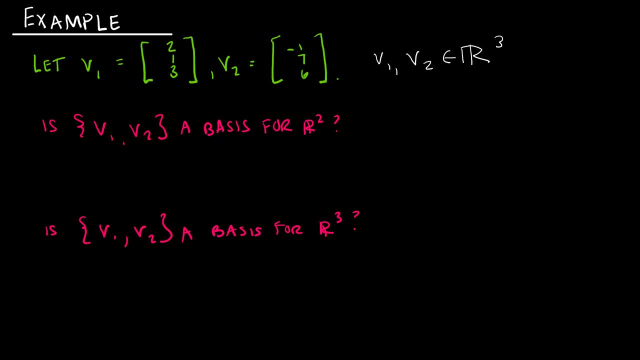 belong to the set R3. There are three entries in each of those vectors. Because they belong to R3, they could not possibly form a basis for R2 because obviously they're not going to span R2.. It's just not going to work. And if you'll recall, our definition previously said that H was a. 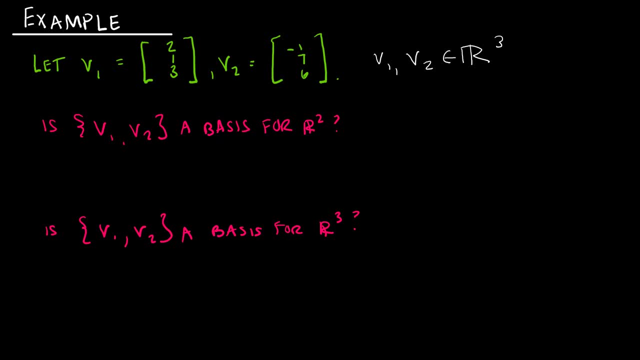 subspace of the vector space and obviously V1 and V2 are not a subspace of R3, which is our vector space in this case. So therefore, no, not a basis for R2.. If I look at R3, I have 2,, 1,, 3, 1, negative. 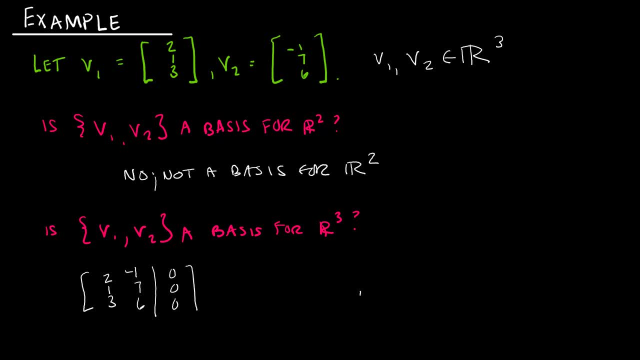 1,, 7,, 6.. And I could do some row operations, but without even doing any row operations, At most I'm going to have two pivots And so not every row has a pivot And therefore this is not going to span R3.. So V1,. 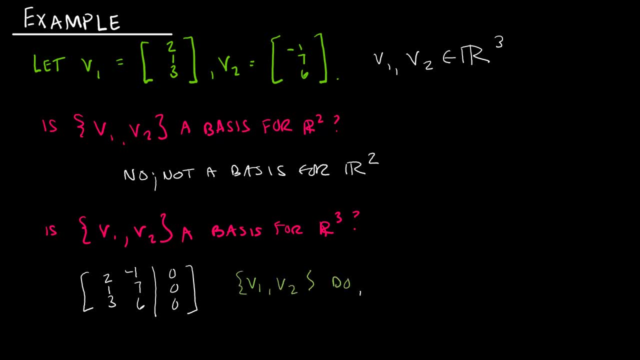 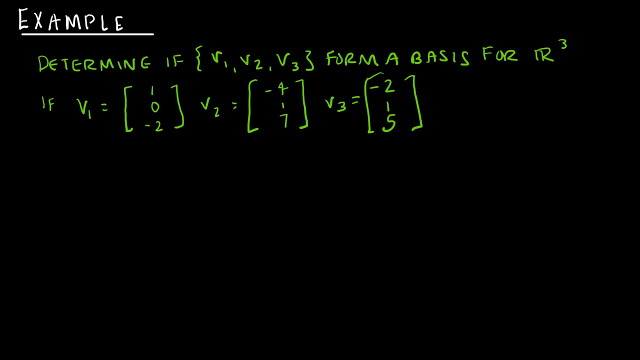 V2 doesn't span R3. And because it doesn't span R3, then we know that this is not a basis by the definition. Here's another example. Again, we're trying to determine if these three vectors form a basis for R3. 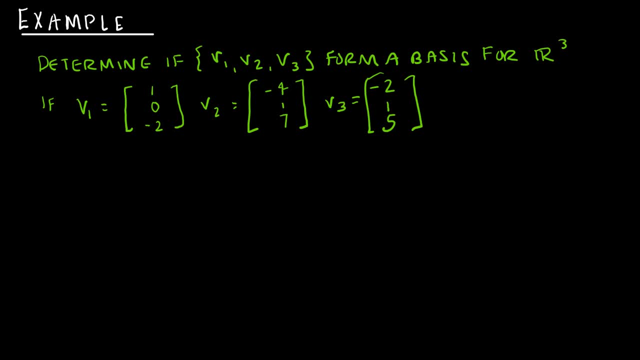 So now I have three vectors in R3, so I have to do a little bit of work. So 1, 0, negative. 2, 4, 1, 7, negative 2, 1, 5.. 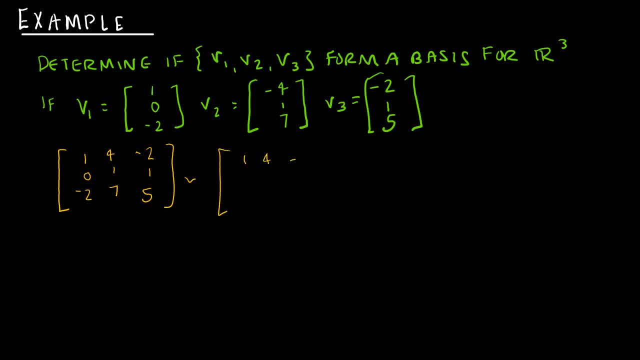 Remember, I'm just going to do row operations to determine if in fact I have a pivot in every row and column, etc. So 0,, 1,, 1.. I'm going to take two times the first row, which gives me 0,, 15,, 1.. And if I keep going I've got 1.. I'm going to take the middle. 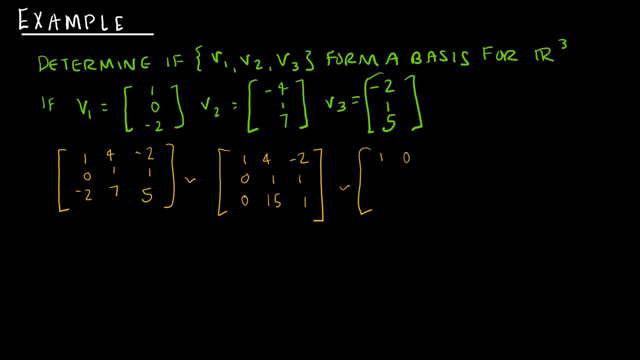 row, row 2, times negative 4, and add it, So that's negative 4 plus negative 2 is negative 6.. Whoops, Row 2, we're keeping just as it is. Row 3, I'm going to take negative 15 times row 2,. 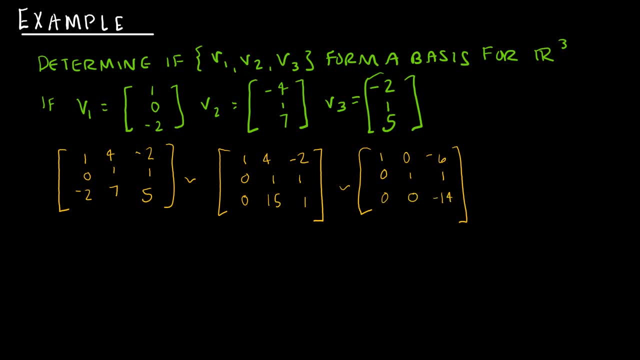 which gives me 0, 0, negative 14.. And from here it's pretty clear that I do in fact have a pivot in each row, and therefore, by the invertible matrix theorem, And again, if I kept going with this, I would get 1, 0, 0, 0, 1, 0, 0, 0, 1.. 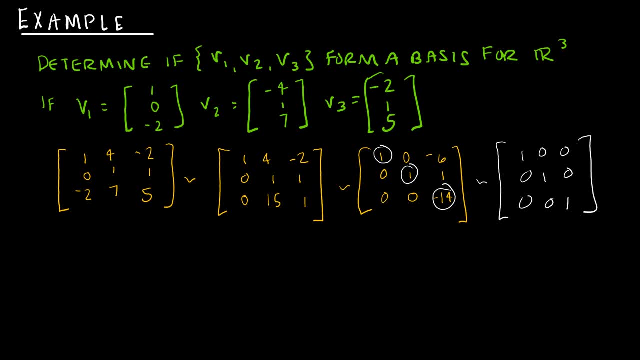 And so what happens then is: this is a basis for R3.. Again, because these row reduced to 0,, I'm sorry- 1, 0, 0, and 0, 1, 0, and 0, 0, 1, which, of course, span R3 and are linearly. 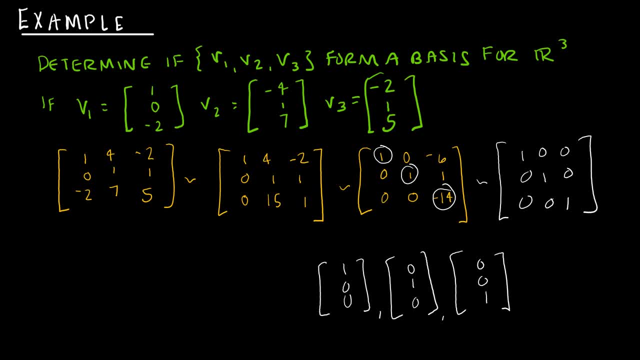 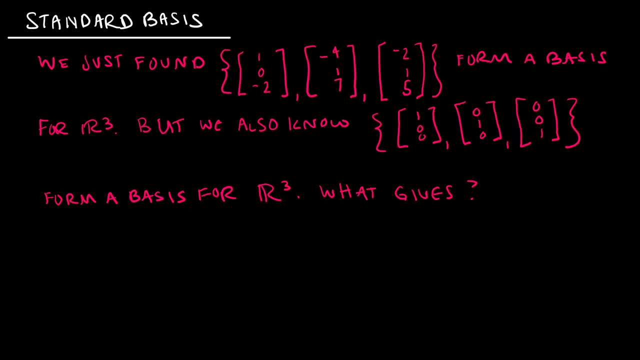 independent. So yes, V1,, V2, V3 do form a basis for R3. And so I'm going to take negative 15 times R3.. In our last example, we found that the vectors I've rewritten here form a basis for R3,. 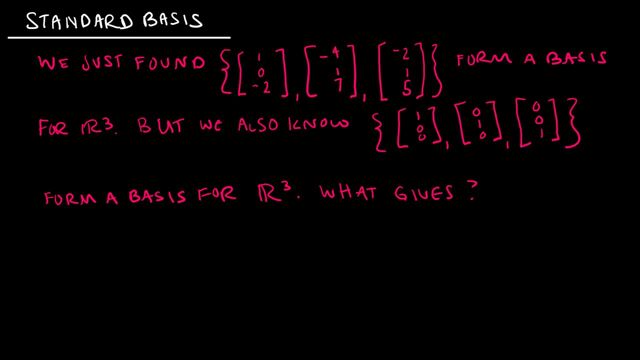 which means they were linearly independent and they span R3.. But we also know that 1, 0, 0, 0, 1, 0, and 0, 0, 1 are vectors that are linearly independent and span R3,. 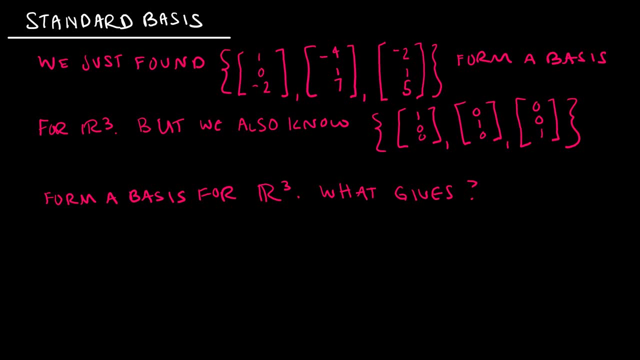 and therefore form a basis for R3.. So what gives? Well, we would call this set of vectors the standard basis. So obviously there are many options for our basis. We could do lots of examples to determine which are basis and which are not, which form a basis and which. 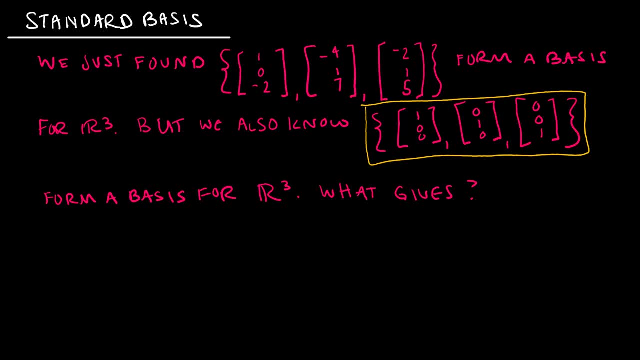 do not, But we know essentially that this is our standard basis. So how did I get there? Remember, when I was looking at my previous example, I did row operations to get it down to reduced row echelon form, And this guy is reduced row echelon form if I put these all together into a matrix.